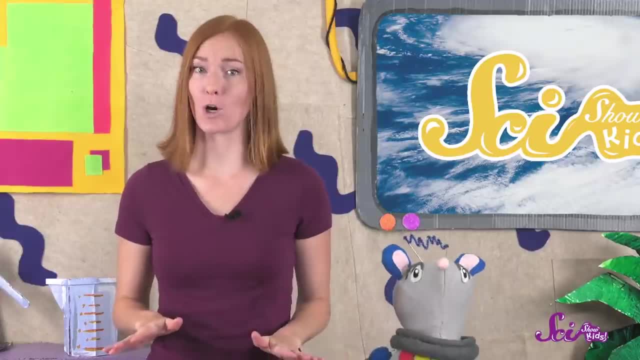 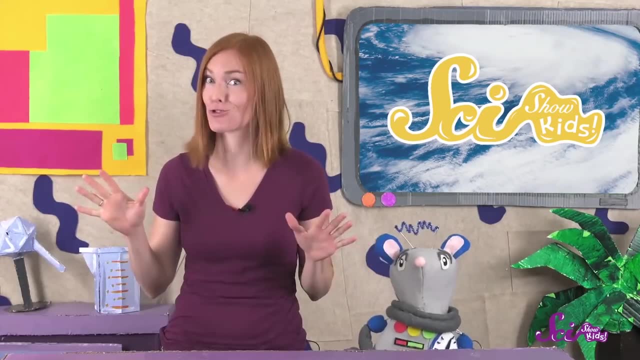 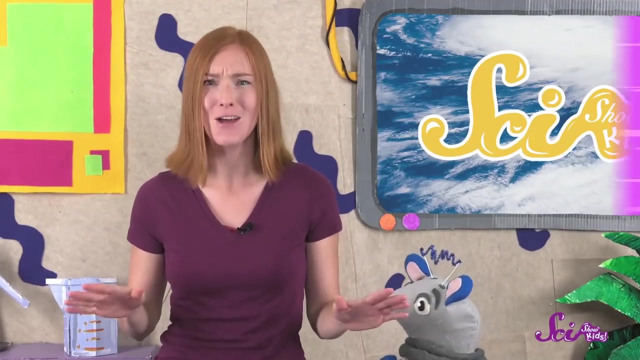 Good thing Squeaks and I have a flashlight just in case, But some areas of the world experience a really extreme kind of storm: a hurricane. Hurricanes are big, powerful storms that have strong winds, And I mean strong. In order to be considered a hurricane, a storm's winds have to be blowing faster than 119 kilometers. 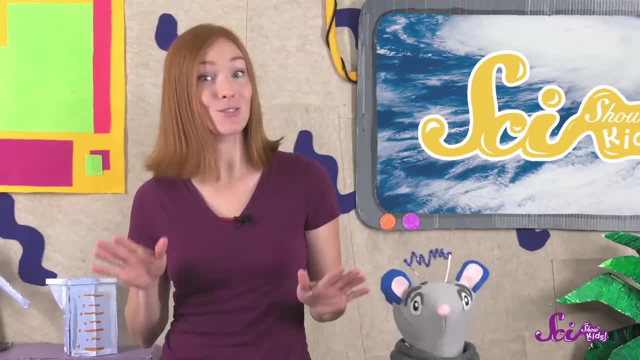 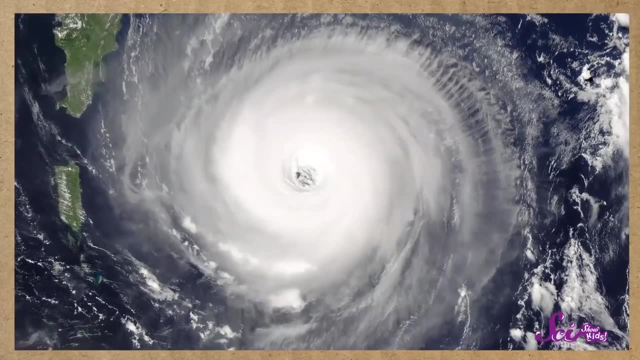 an hour. That's faster than a car zooming down the highway. Sometimes you'll also hear this kind of storm called a cyclone or a typhoon, but they're all just different names for the same thing. From space, many hurricanes look like this: big, swirling storms that have a really cool 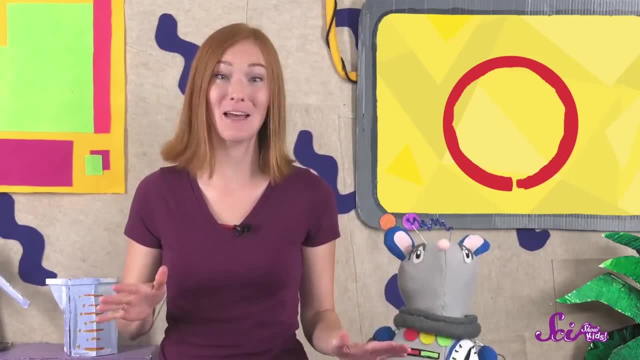 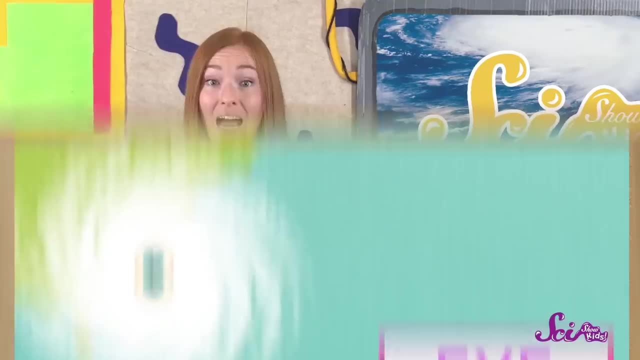 shape- That's right- Squeaks. This hurricane looks a little bit like a circle. The clouds wind around a space in the center of the hurricane called the eye. It even sort of looks like an eyeball. Now, a hurricane's shape is pretty cool, but it's not the only thing that's special. 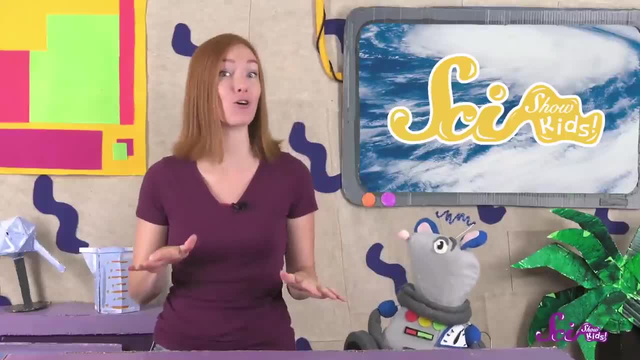 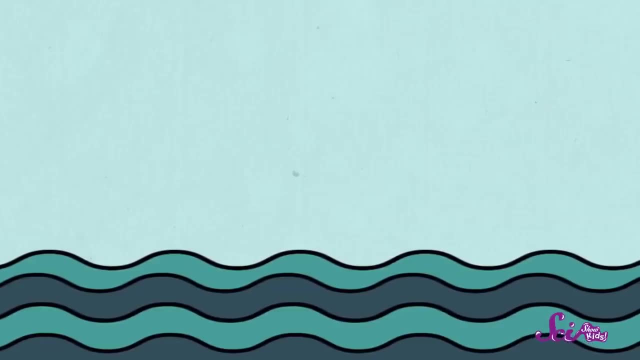 about this kind of storm. Everything has to be just right for a hurricane to form. It's kind of like a puzzle. The first piece of the hurricane puzzle is warm ocean water. The water has to be at least 27 degrees Celsius or about as warm as a swimming pool. for a 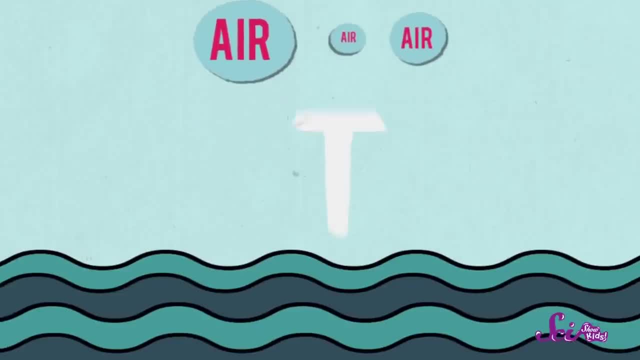 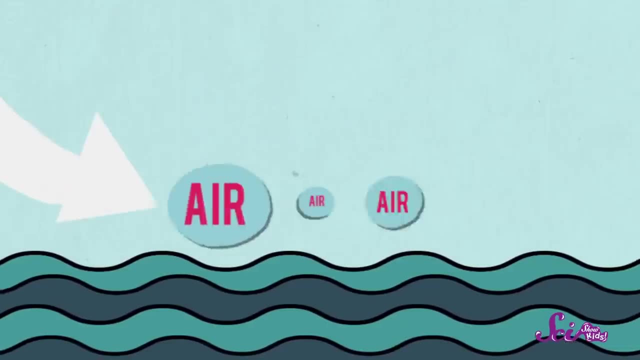 hurricane to form. The warm water causes the air above it to warm up and rise high enough to cover the sky. The warm air is very humid, which means that there's a lot of water in it. As the air rises into the sky, other air rushes in to take its place. 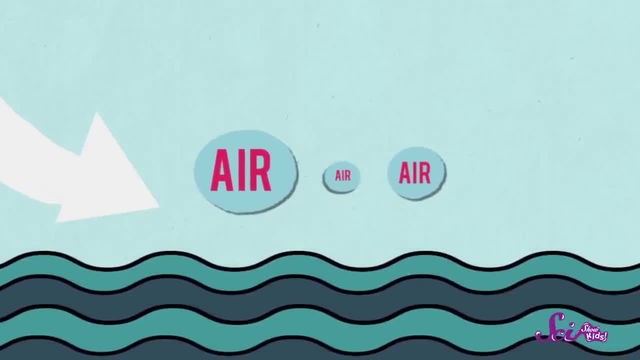 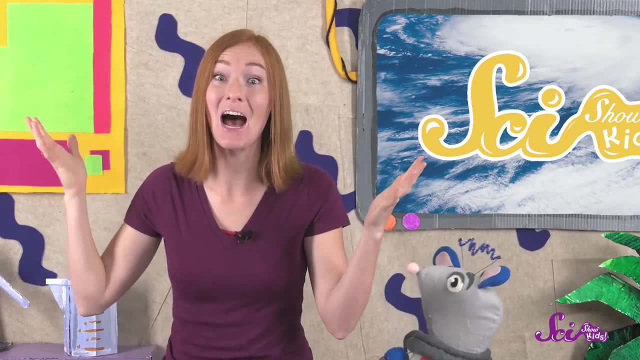 The air that rushes in gets warm and humid too, and then it rises high into the sky as well. As the air rises, it cools and clouds start to form- Lots of them. High in the sky is also where we find the second thing that's important for making. 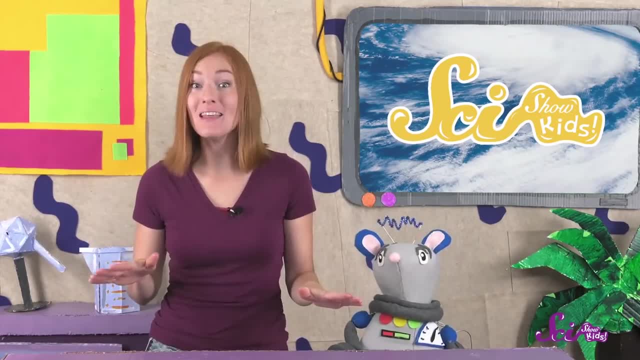 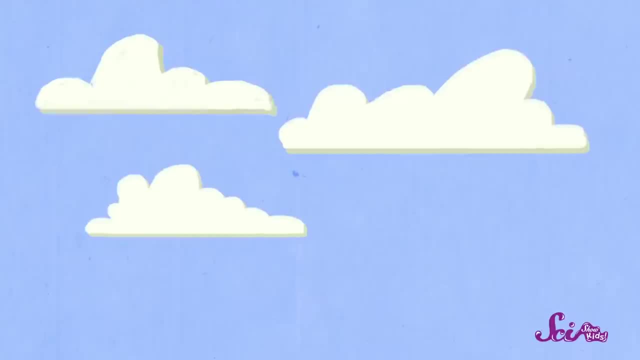 a hurricane — wind, And not just any wind. The wind that helps make a hurricane has to be calm and steady. It can't be the kind of wind that blows really hard for a moment or two and then calms down again. If there are sudden gusts like that, the storm can get blown apart, kind of like how a candle. gets blown out. But if there's warm, damp air along with those steady winds and it stays like that for a few days, the rest of the pieces that make up a hurricane fall into place. The steady winds push the growing storm over the ocean and the warm water gives the storm. energy. It causes more air to rise, more clouds to form and the winds inside the hurricane become stronger. In fact, the only place that it's not very windy is in the hurricane's eye. It's actually very calm in the eye, even though it's right in the middle of the storm. As it grows the hurricane also starts to turn. It spins around with the eye in the center, kind of like a top. As long as hurricanes have that warm air for fuel, they can keep going and keep growing. But when they reach land or pass over cooler water they lose their warm air. so they start. to fall apart. That's why hurricanes are so strong. They're so strong, They have a lot of rain, though Sometimes the rain can last for days. They also can push a lot of ocean water onto the shore, which can cause a lot of floods. But people can prepare for hurricanes, especially if they know when they're going to happen. For example, most hurricanes near North America happen between May and November every year because that's when the different pieces that make a hurricane fit together the best And scientists have lots of tools to try and track hurricanes.